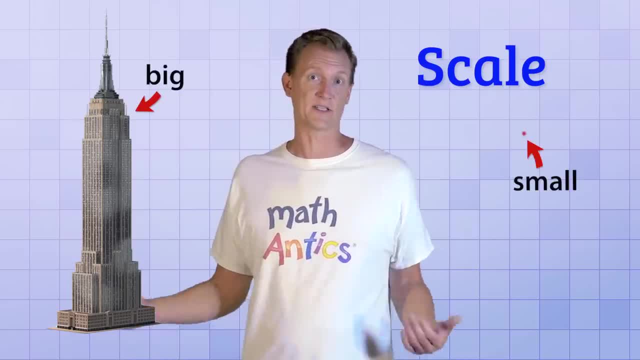 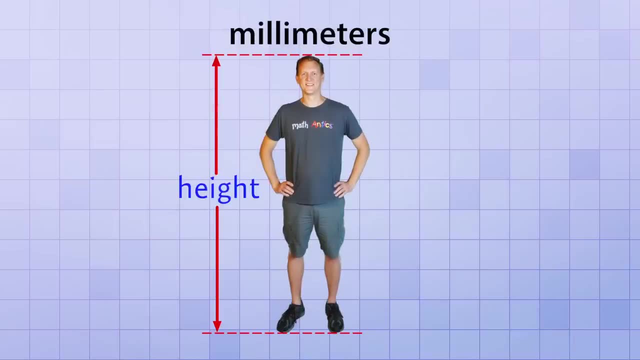 to choose a unit of measurement that's a good match for a particular object's scale. Here's what I mean by that. Suppose I decide to measure my height using millimeters, which are really small units about the size of an ant, I would be about 1980 millimeters tall. 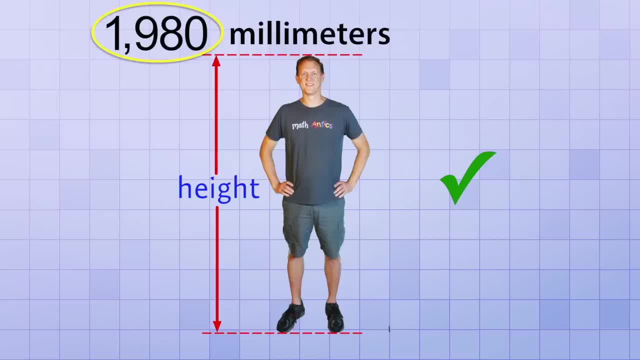 And while that's a correct measurement, it's kind of a big number that makes me seem even taller than I really am. On the other hand… If I decide to measure my height using a really big unit like kilometers, I'd be a mere. 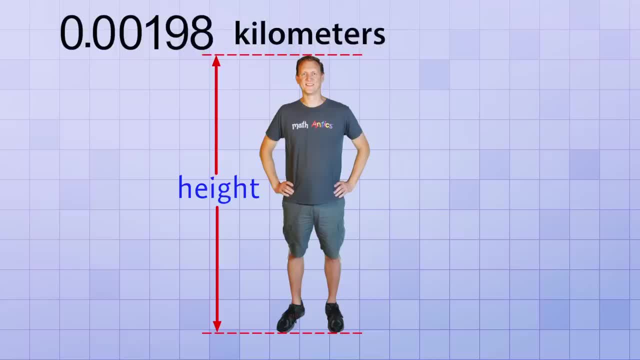 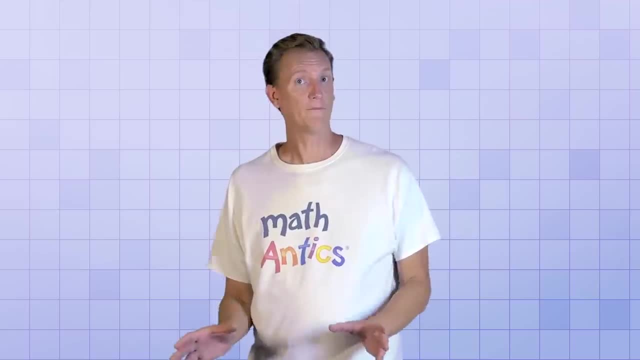 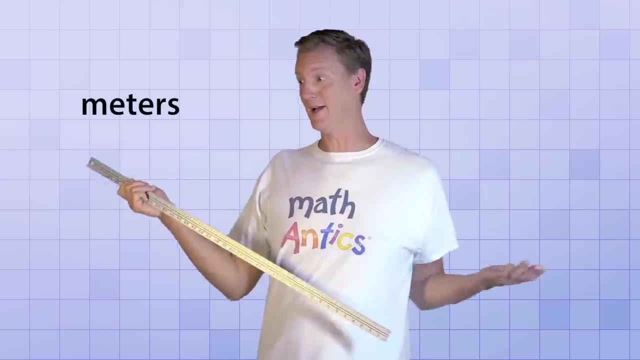 0.00198 kilometers tall. Again, that's a correct measurement, but it's a really small number that makes me seem tiny. But what if I choose a unit that's somewhere in between, like plain ol' meters? A meter is as long as this stick, which is why I like to call it a meter stick. 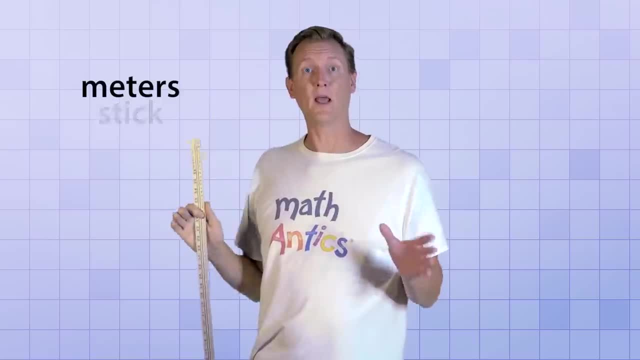 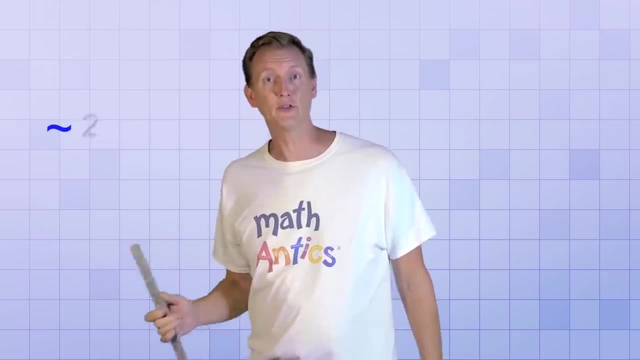 And if I use it to measure my height… I'd be 1.98 meters tall, Which is just a hair shy of 2 meters. So it would be fair to say that I'm about 2 meters tall, which is a nice easy number. to work with. See the advantage of having different sized units for measuring distances. You can choose a unit that's relatively close to the scale of the thing that you want to measure, so that the numbers you get are more relatable and easy to work with. 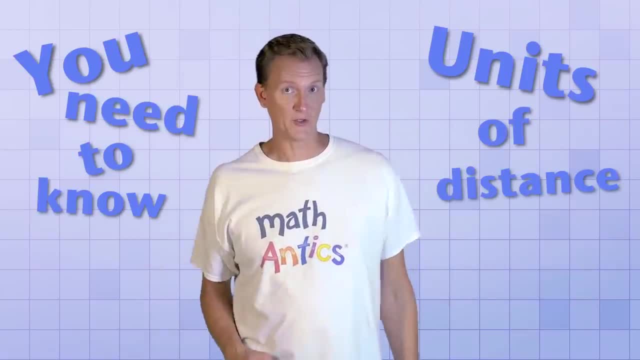 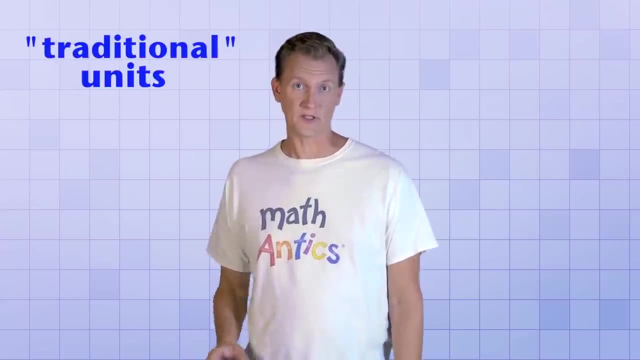 But that means that you need to know about the different units of distance so you can make a good choice, right? So that's what we're going to focus on in the rest of this video. Specifically… We're going to learn about 4 traditional units that are still used in America for measuring. 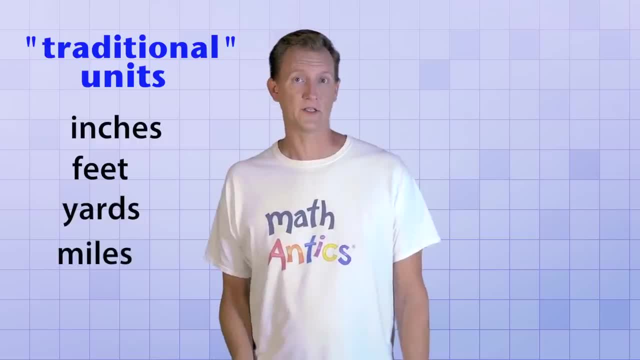 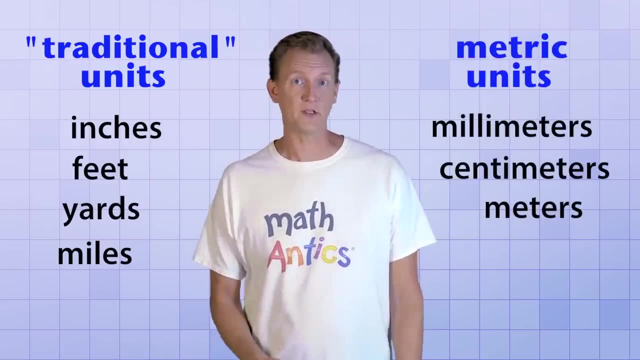 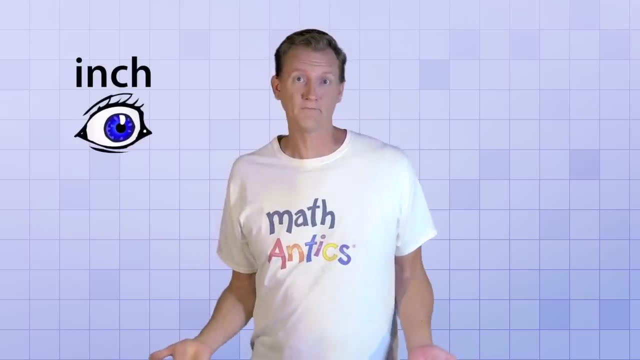 distances- Inches, feet, yards and miles- And then we'll see how those compare to the 4 most popular metric units for measuring distance: Millimeters, centimeters, meters and kilometers. Let's start with an inch. An inch is about this wide, which is pretty close to the width of a human eye. 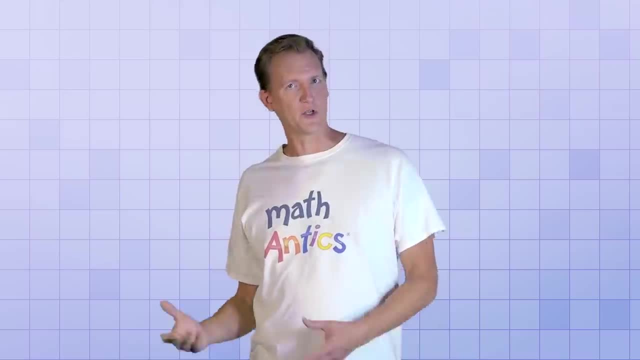 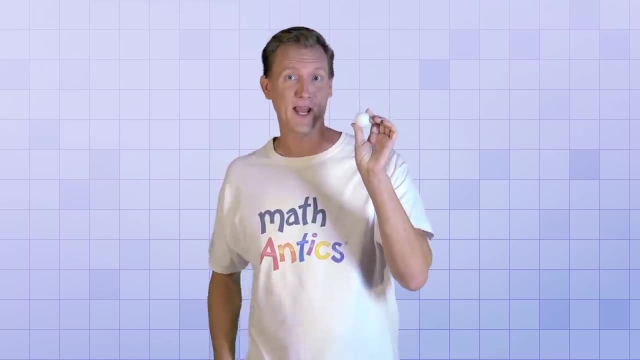 Or perhaps the width of your thumb if you have big fingers. An inch is a good sized unit for measuring objects that we commonly interact with. For example… My ping pong ball is about 1 and a half inches in diameter And my phone is about 6 inches tall. 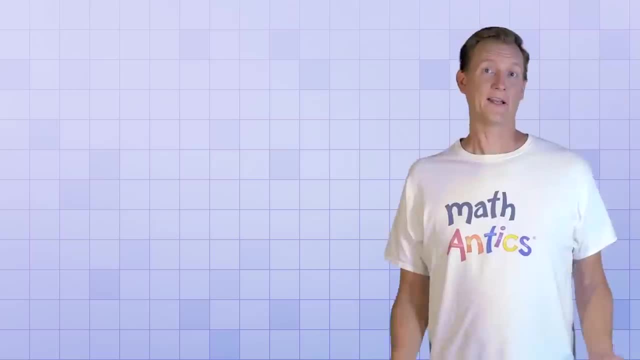 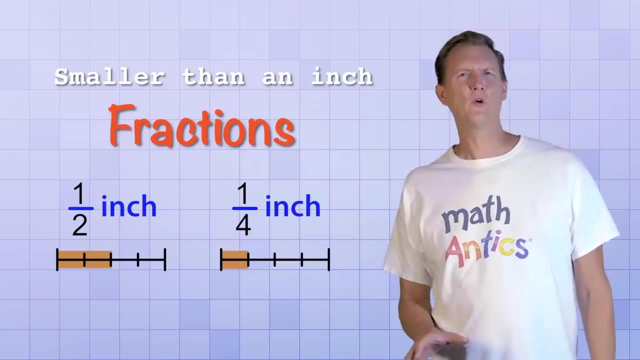 And an unsharpened pencil is about 8 inches long, And it's common to measure things that are smaller than an inch using fractions like a half inch or a quarter inch. We'll learn more about fractions of an inch in a future video, when we talk about measuring. 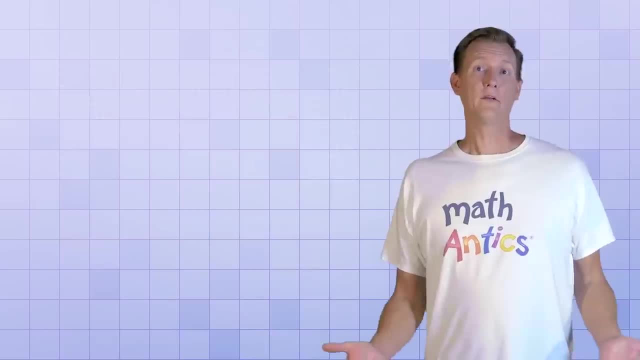 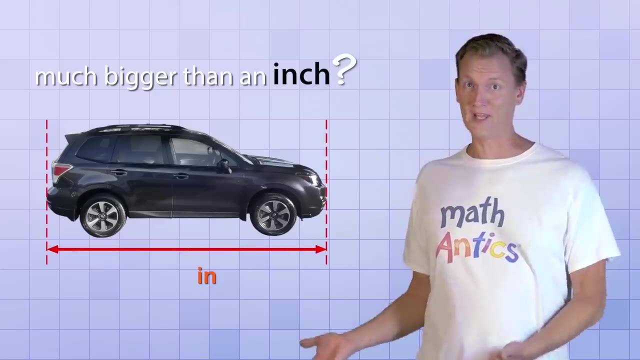 devices like rulers and tape measures, OK. but what if we want to measure things much bigger than an inch, like a car? Well… We can either use inches and just end up with a big measurement, Or we can use a bigger unit called a foot. 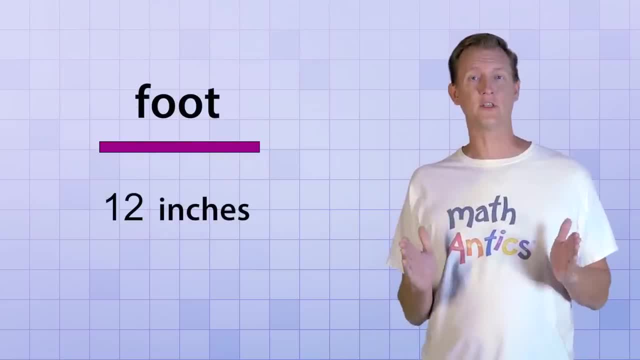 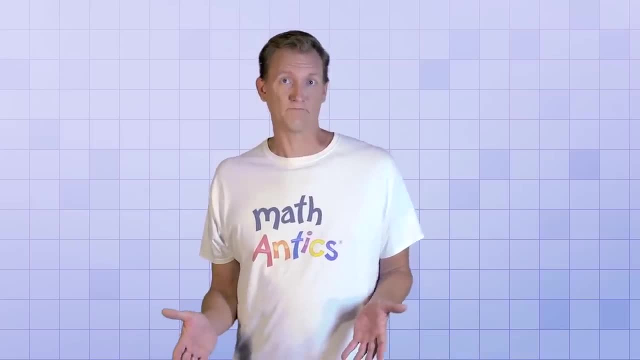 A foot is exactly the same distance as 12 inches stacked end to end, So it's about this long. Some familiar objects that are approximately a foot long are well your foot, for one thing. Of course, different people have different sized feet. 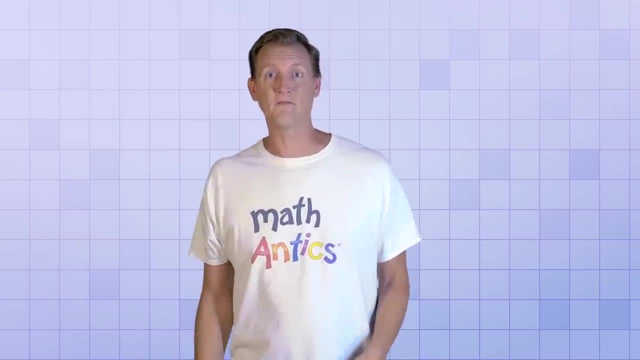 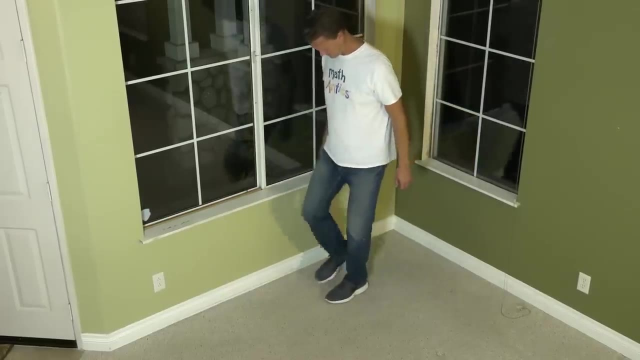 And most people have feet that are less than a foot long, But the length of the average shoe is a pretty good estimate for a foot …. And that's why you'll sometimes see people walking off a distance heel to toe to estimate how many feet that distance is. 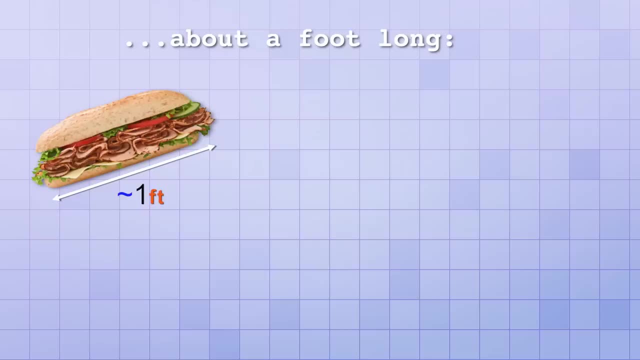 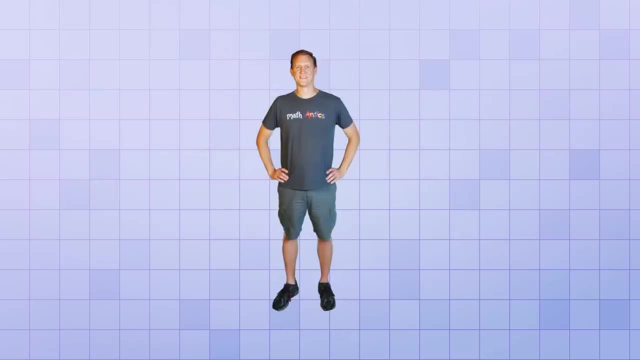 Other things that are about a foot long are a foot-long sub sandwich, a tall water bottle or a three-ring binder, And a foot is a convenient unit for measuring things like a person's height. I happen to be 6 and a half feet tall. 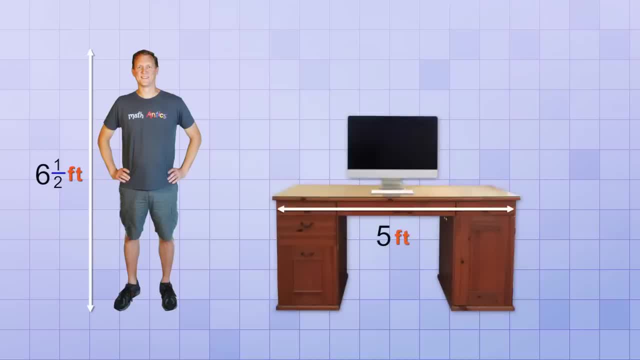 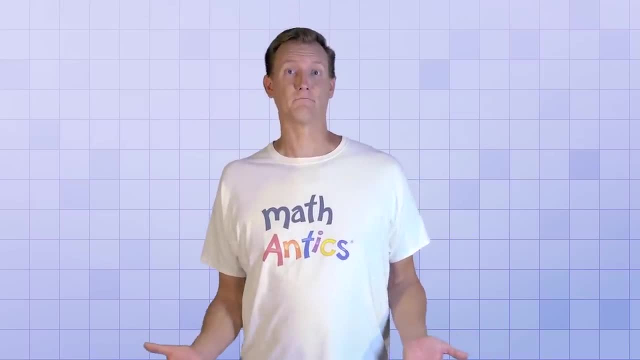 Or the width of a desk: Mine's about 5 feet wide. Or the length of a car: Mine's about 15 feet long. All right, What about something much bigger than a foot, Like an athletic field? Well, that's what a yard is for. 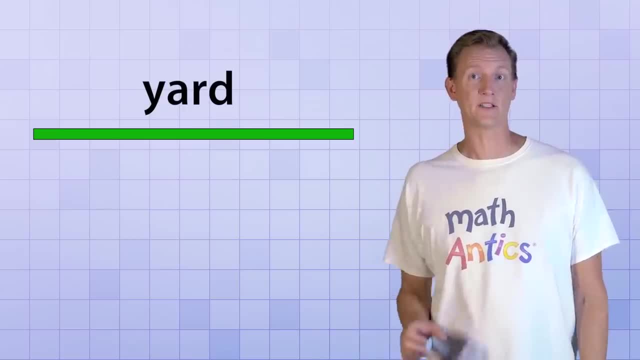 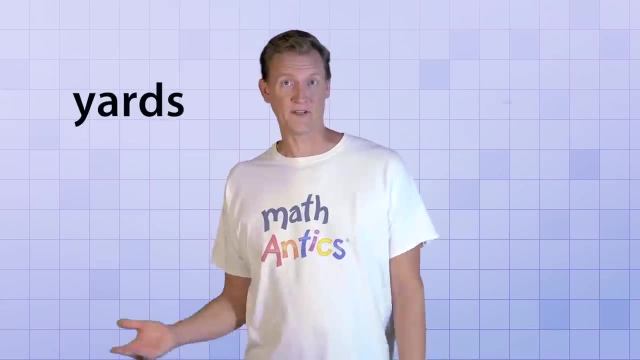 A yard is an English unit of measurement. that's exactly the same as three feet placed end to end, So a yard is about this long. In general, yards aren't used as often as feet, But one place where yards are used all the time is in American football. 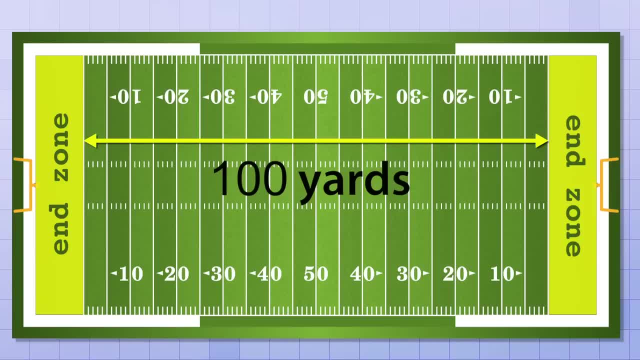 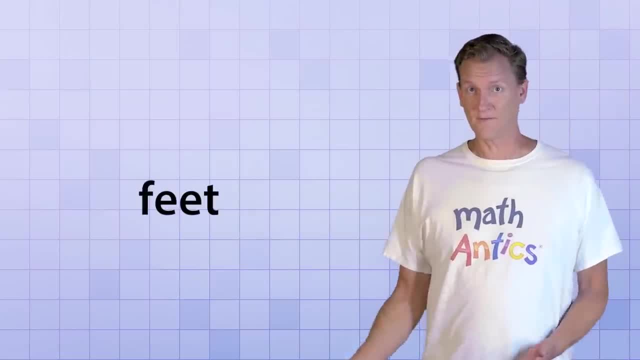 Between the end zones, an American football field is 100 yards long, And those 100 yards are divided into subgroups of 5 yards each. So you can measure some pretty big distances with feet and yards. But what if you need a unit that's even bigger? 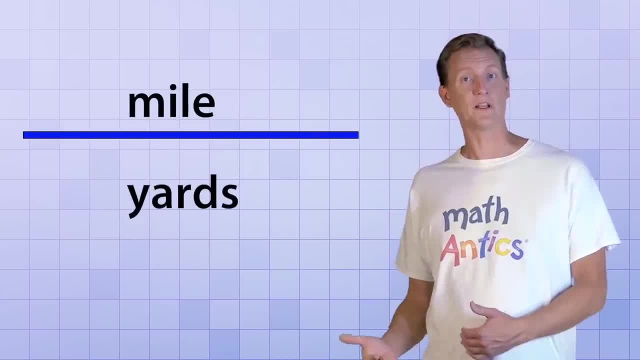 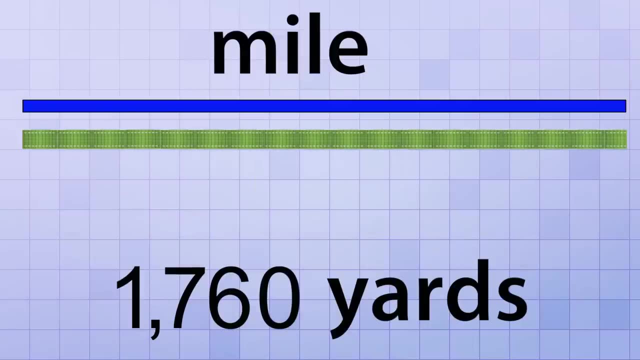 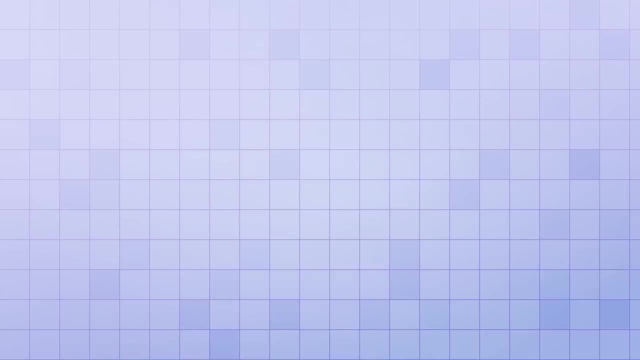 Well, that's where miles come in handy. A mile is equivalent to 1,760 yards. That's the distance you would get if you put 17.6 football fields end to end, Which is pretty far. A mile is much bigger than the other three units we've looked at so far. 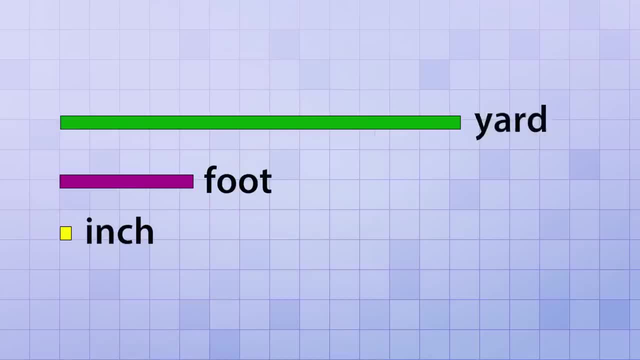 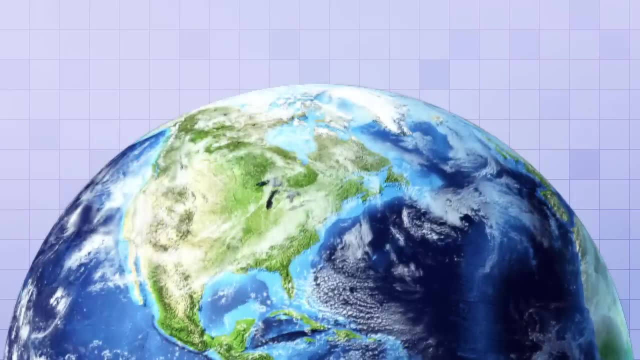 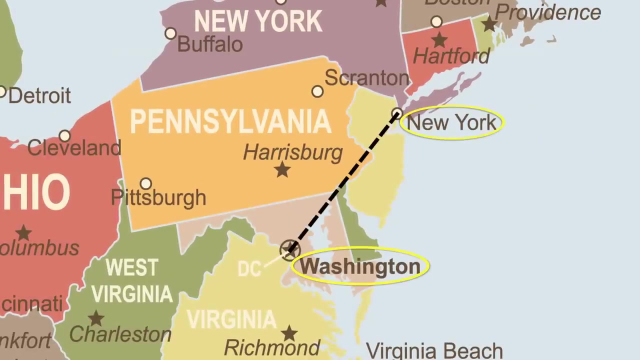 If this is an inch, then this is a foot and this is a yard, then this is a mile. Because miles are so long, they're mainly used to measure distances between various places on Earth and how far people travel. For example, the distance from New York City to Washington DC is roughly 200 miles as the crow flies. 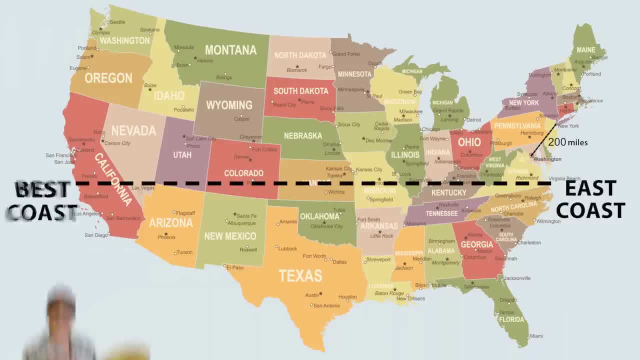 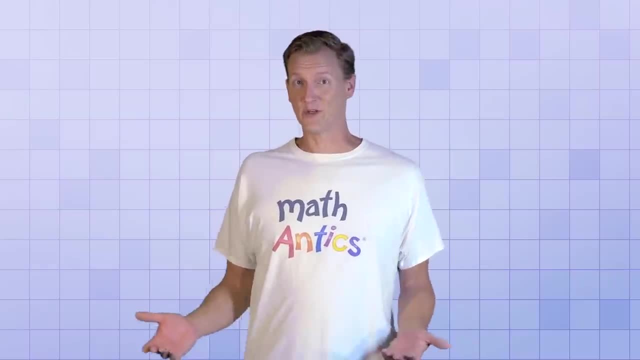 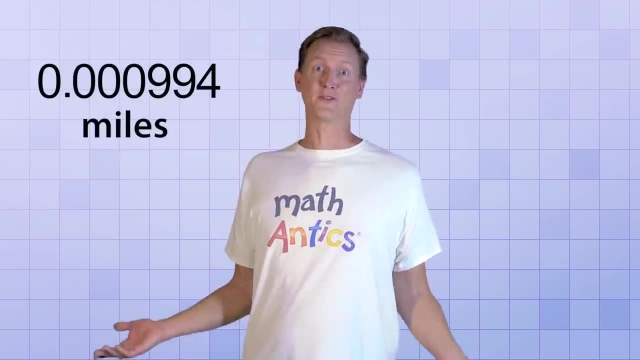 And the distance from the east coast of the US to the west coast, or the best coast, whichever you like to call it, is over 2,600 miles. Sure, you could use miles to measure smaller distances, but it'd be a little silly to tell your friend that you're 0.000994 miles tall. but go ahead if you want to. 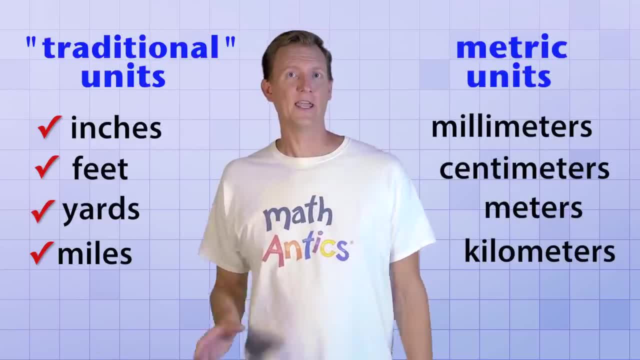 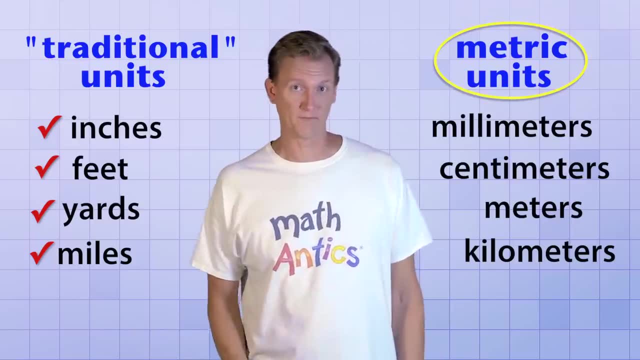 Okay, so that takes care of the four main traditional units. Now let's have a look at the four most common metric or SI units of distance which are preferred by the scientific community and most countries. We're going to start with a unit called a centimeter. 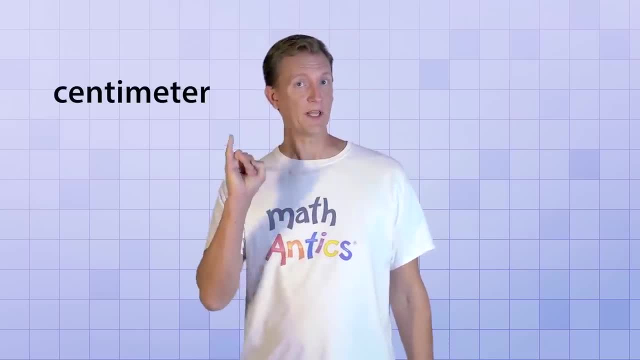 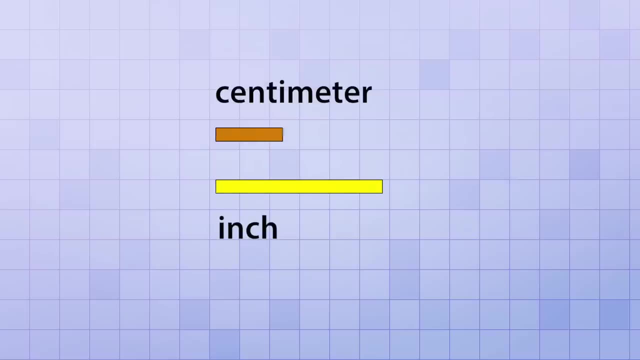 A centimeter is pretty small. It's approximately the width of your pinky finger or the diameter of your pinky finger of a small marble. If you compare a centimeter to an inch, you'll find that it takes about two and a half centimeters to equal one inch. 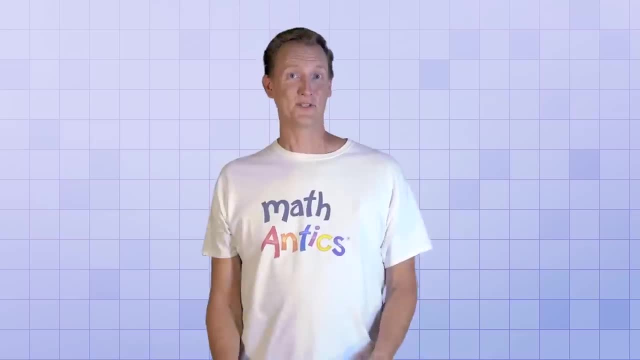 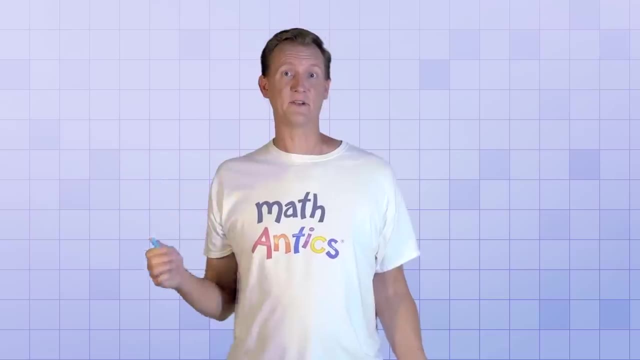 2.54 centimeters to be exact, So centimeters are also really good units for measuring objects that you commonly interact with. This rechargeable battery is about five centimeters long. This tennis ball is about six and a half centimeters in diameter. 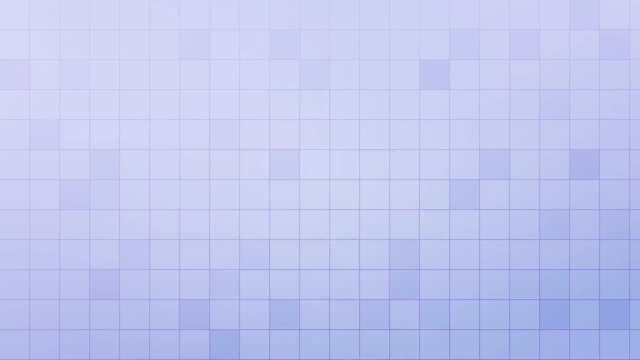 And this flashlight is nearly 23 centimeters long, Wow. But what if you want to measure things that are smaller than a centimeter? Well, you could measure things that are smaller than a centimeter. Well, millimeters might be a good choice. 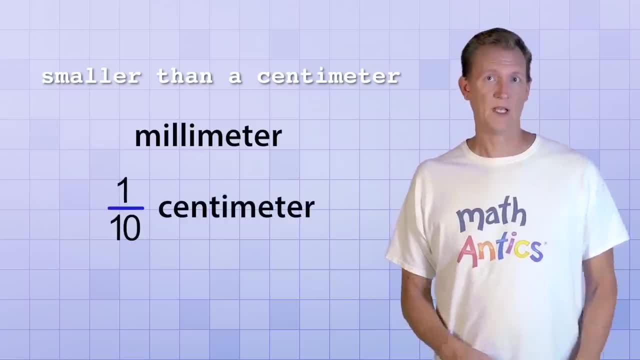 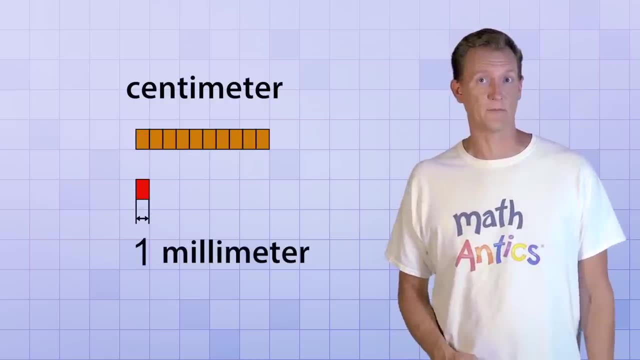 A millimeter is exactly one-tenth of a centimeter. That means if you took a centimeter and divided it up into ten equal parts, each of those parts would be the distance of one millimeter. A millimeter is about the width of a small black ant. 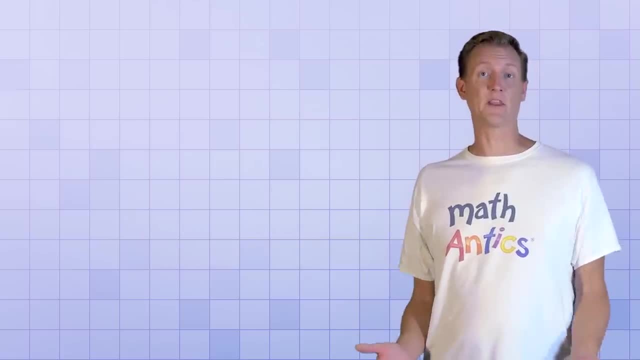 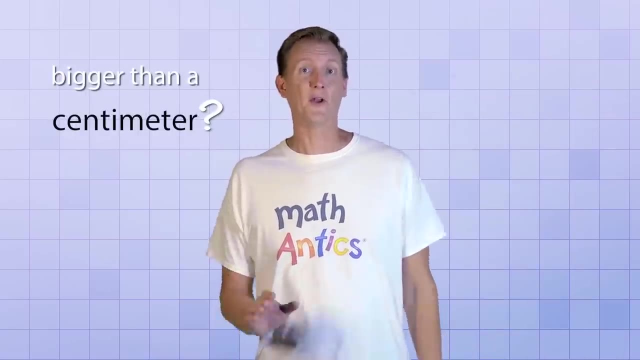 So millimeters are good for measuring small things like the width of a sunflower seed or the thickness of a smartphone. Okay, but what if we need to measure something bigger than a centimeter? No problem, We can just use meters. 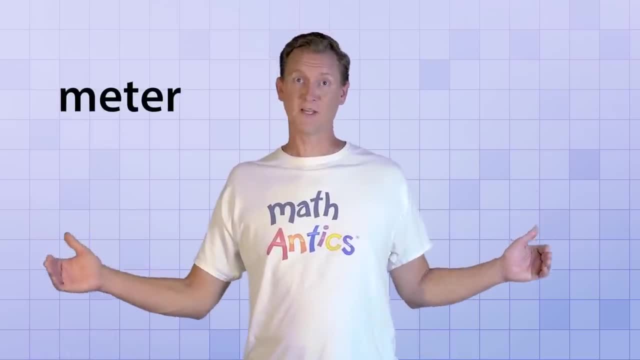 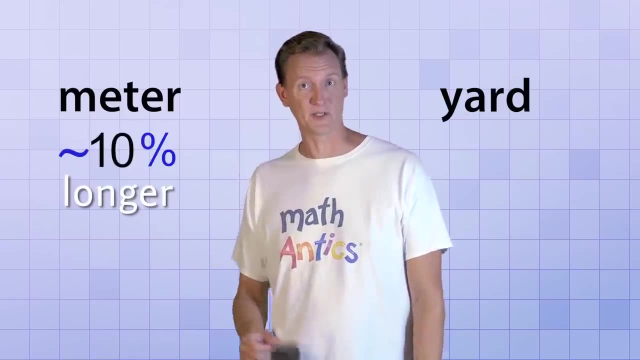 A meter is a unit of distance. that's about this long. That looks similar in length to a yard, doesn't it? It turns out that a meter is just a little longer than a yard, Approximately 10% longer. But the important thing to know about a meter is that it's the exact distance you'd get. 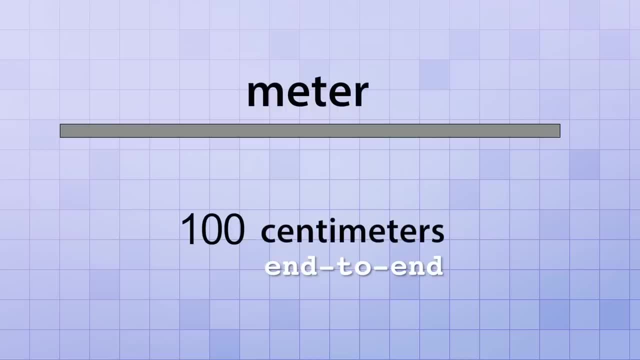 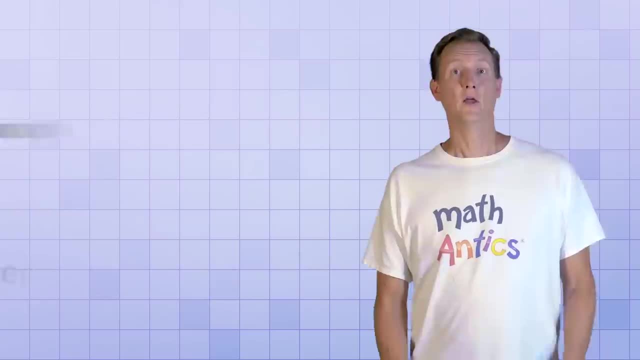 if you took 100 centimeters and placed them end-to-end, Yep, 100 centimeters equals one meter, which means that a centimeter is one-one-hundredth of a meter. Meters are great for measuring distances like the height of a building. 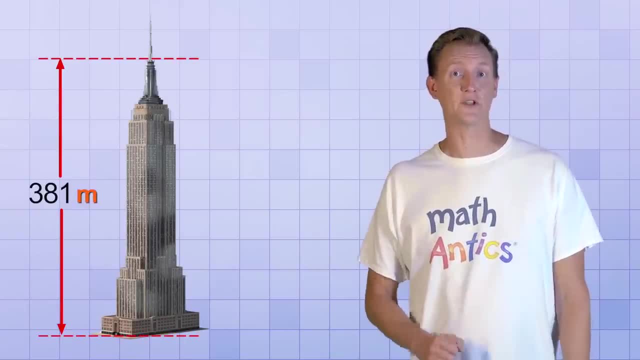 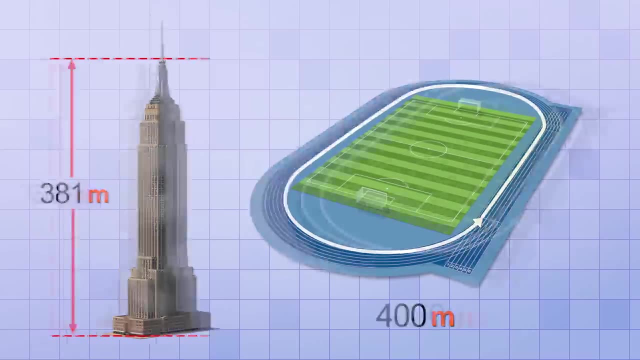 This one is 381 meters tall, Or the distance around a racetrack, which is 400 meters. But if you needed to measure even longer distances, you could use kilometers or kilometers. A kilometer is the distance you'd get if you took exactly 1,000 meters. 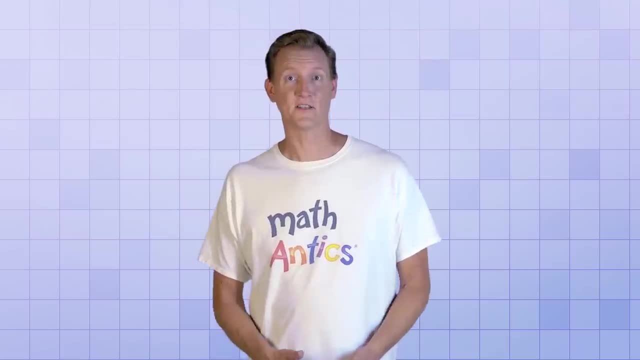 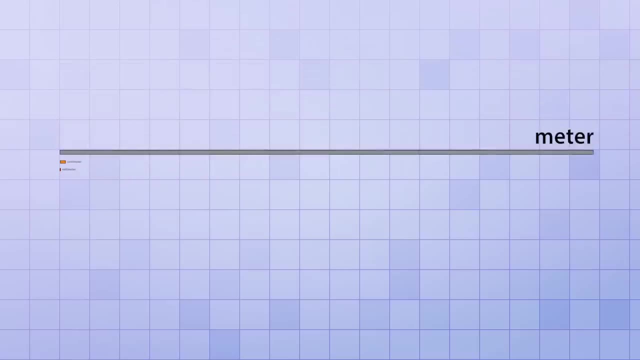 and placed them end-to-end. That's a long distance. It's much longer than the other metric units we've seen. If this is a millimeter, this is a centimeter and this is a meter, then this is a kilometer. As you can see, a kilometer is in the same scale range as a mile, But a mile is even longer than a kilometer. In fact, it takes just a bit more than 1.6 kilometers to be the same distance as a mile. 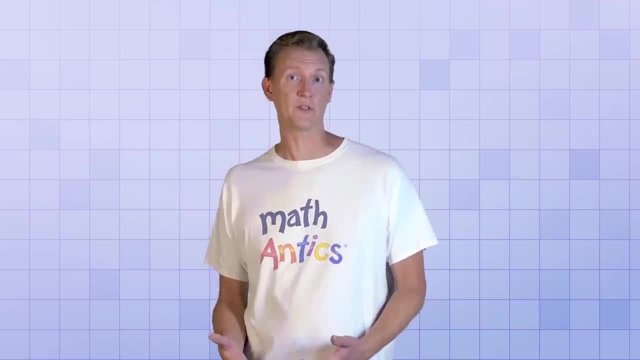 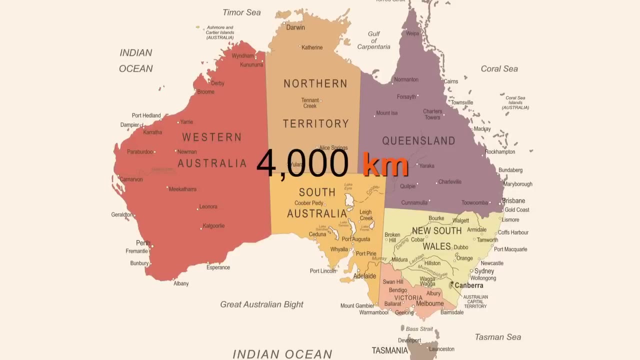 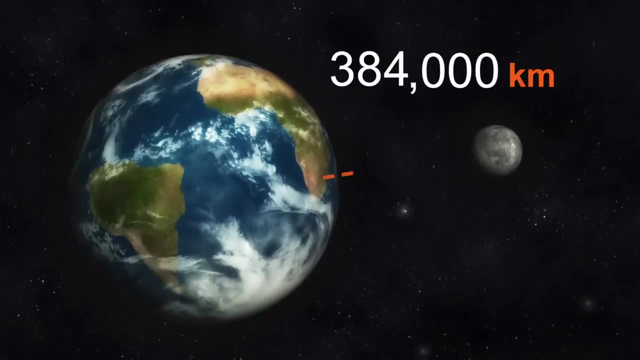 And because they're big like miles, kilometers are also primarily used to measure distances between different locations on the Earth or even in space. For example, it's about 4,000 kilometers from the east coast of Australia to the west coast, And it's approximately 384,000 kilometers from the Earth. 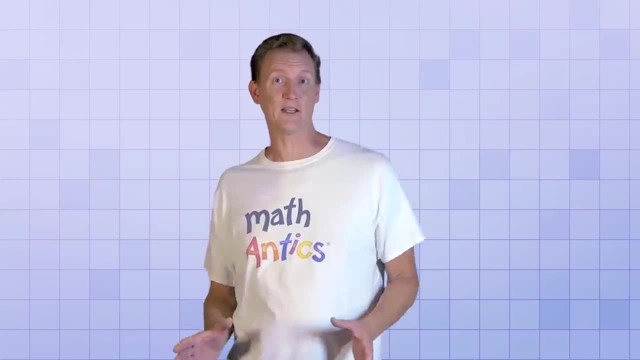 to the moon. Okay, so now that you have a better idea about the size of the most common traditional and metric units of distance, let's do some side-by-side comparisons so you get a better feel for how these units relate to each other. 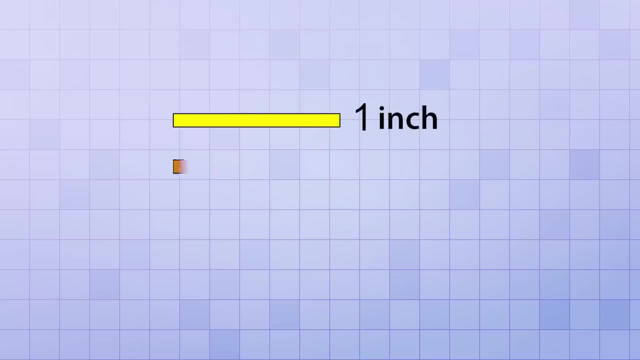 Again, let's start with an inch. We already learned that an inch is the same distance as 2.54 centimeters, right? So how many millimeters would be equal to an inch? Well, since there's exactly 10 millimeters in each centimeter. 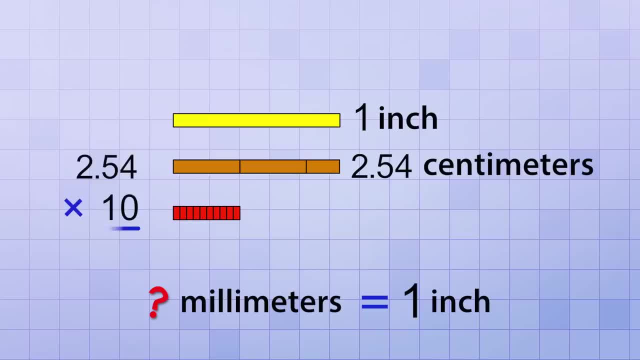 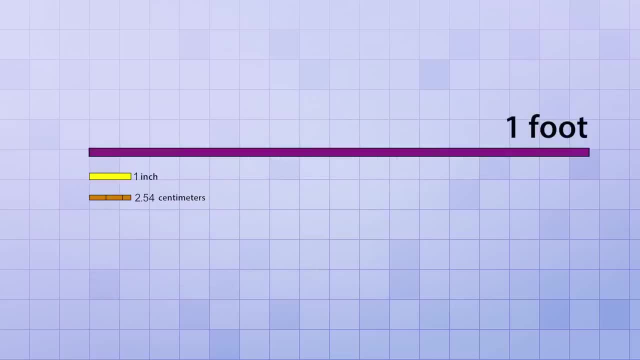 all we have to do is multiply 2.54 by 10, and we see that there are 25.4 millimeters in an inch. But now let's bring in a foot. We know that there's exactly 12 inches in a foot. 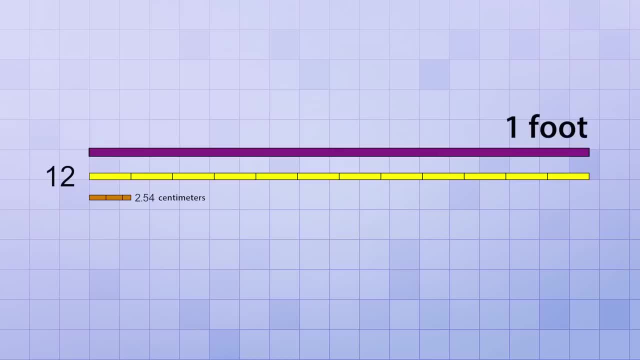 which means that a foot is 12 times longer than an inch. So how many centimeters are there in a foot? Well, since there's 2.54 centimeters in an inch, if we multiply that by 12, we'll know how many centimeters are in a foot. 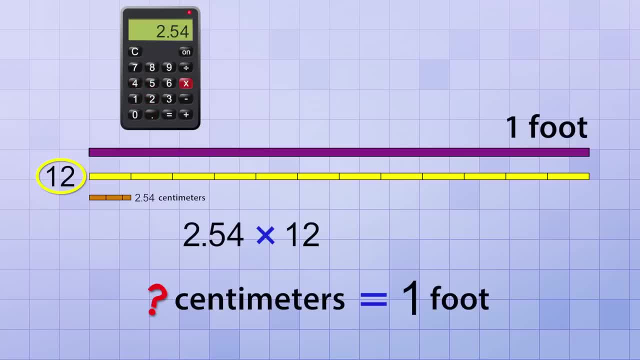 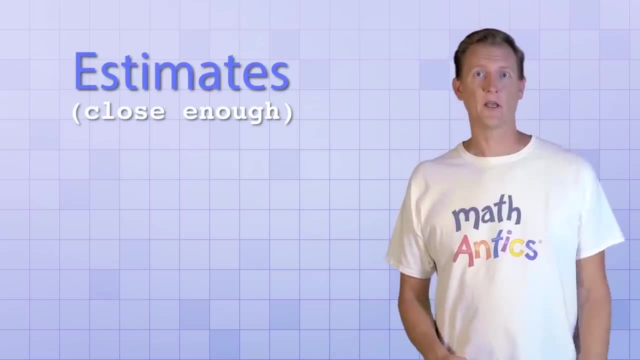 Using my trusty calculator, 2.54 times 12 equals 30.48.. So a foot is exactly 30.48 centimeters long. Those are exact conversions between inches, centimeters and feet. But what if you only need estimates or close enough measurements? 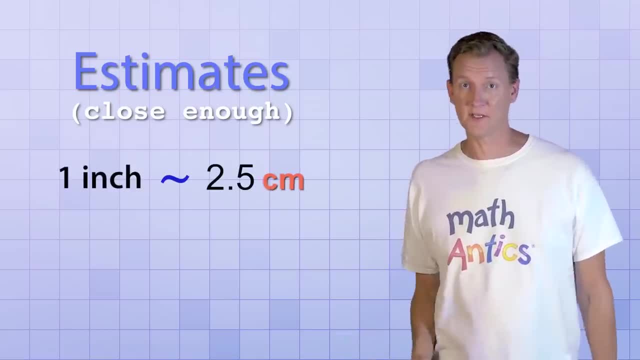 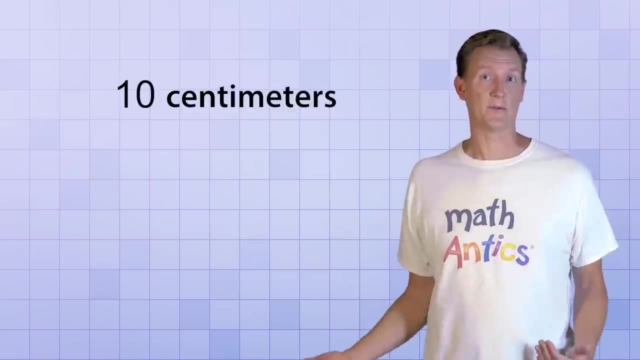 In that case, just remember that an inch is about 2.5 centimeters and a foot is about 30 centimeters. Let's do another quick comparison, starting with 10 centimeters instead. If you have 10 centimeters, it's easy to see that it's equivalent to 100 millimeters. 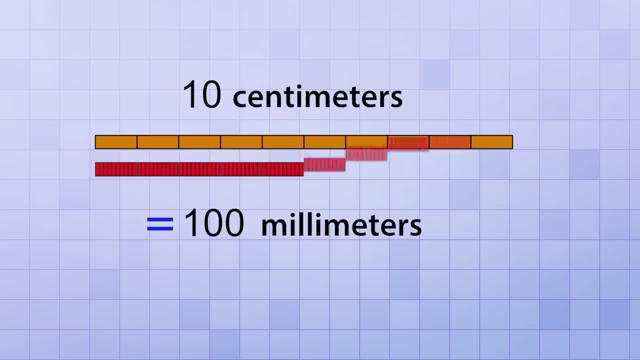 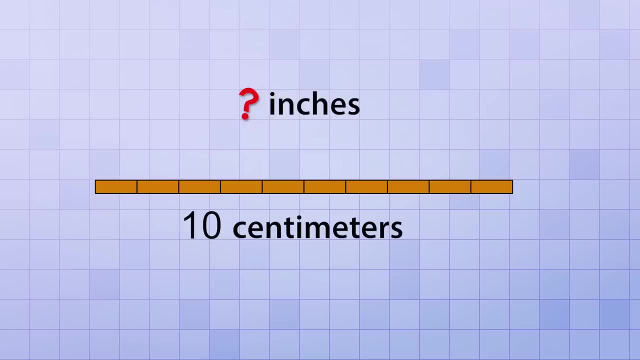 since there's 10 millimeters in every centimeter. 10 times 10 equals 100. But what would that same distance be in inches? Well, an inch is bigger than a centimeter, and it takes approximately 2.5 centimeters to equal an inch right. 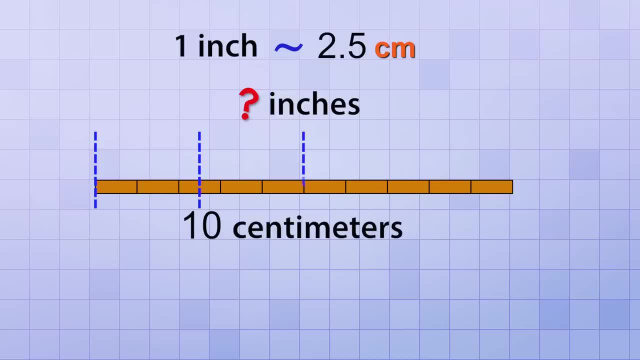 So if we divide the 10 centimeters up into groups of 2.5, which is the same as dividing 10 by 2.5, it forms 4 equal-sized groups. That means 10 centimeters is very close to being the same as 4 inches. 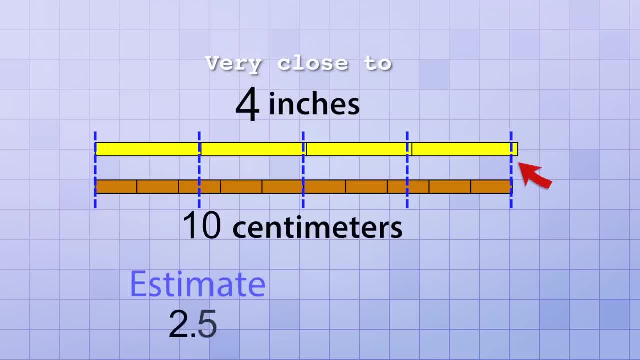 The reason it's only very close is because we used the estimate 2.5 centimeters per inch instead of the exact value of 2.54.. If we divided 10 by 2.54 instead, we'd see that 10 centimeters is more like 3.937 inches. 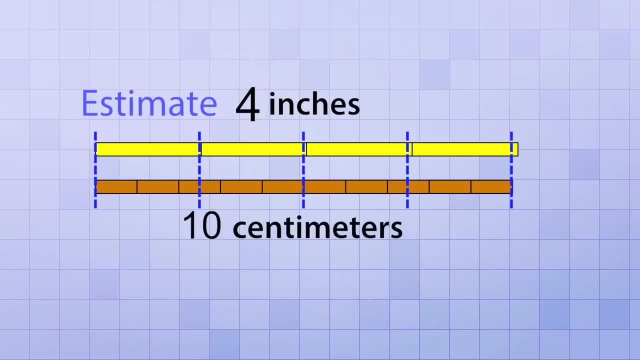 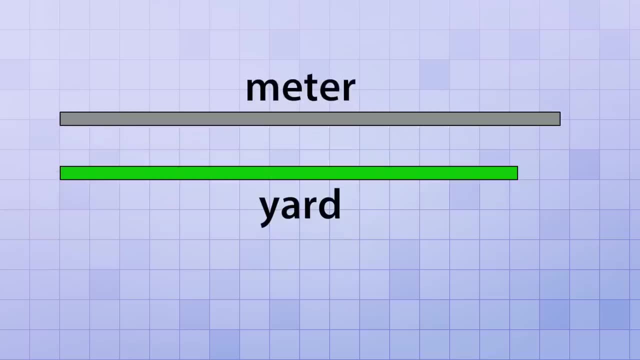 But 4 is a great estimate and it's easier to remember. 10 centimeters is about 4 inches. Now that we've compared some of the smaller units, let's briefly look at the bigger ones. We learned that a meter is about 10% bigger than a yard. or roughly 1.1 yards. That's a good estimate, but more precisely to three decimal places, a meter is 1.094 yards. A yard is 3 feet, so that means a meter is a little more than 3 feet. 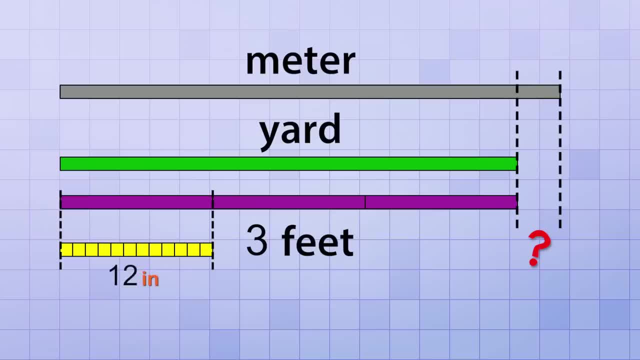 How much more? Well, each foot in a yard is 12 inches, so a yard is 36 inches, since 3 times 12 equals 36.. Our estimate is that a meter is 10% bigger than a yard. So what's 10% of 36 inches? 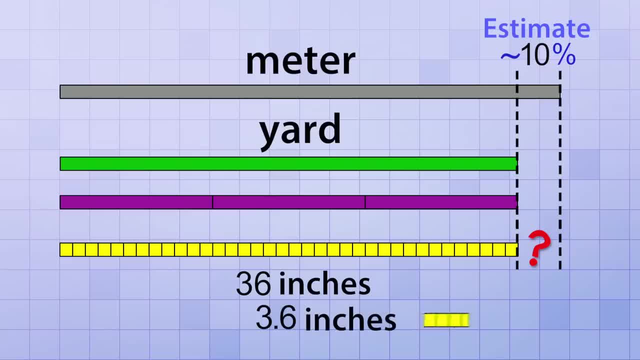 Yep, 3.6 inches And if we add that to 36 inches that means a meter is pretty close to 39.6 inches or 40 inches if we round up a little And that checks out, because remember.